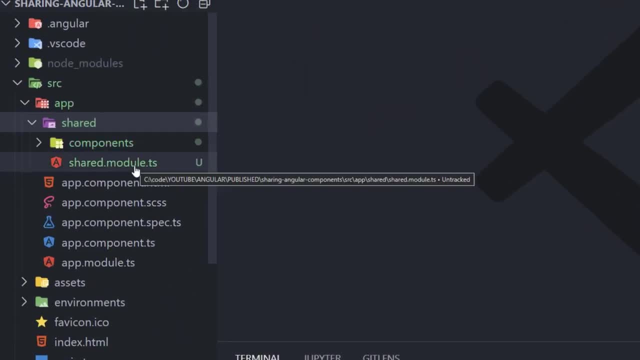 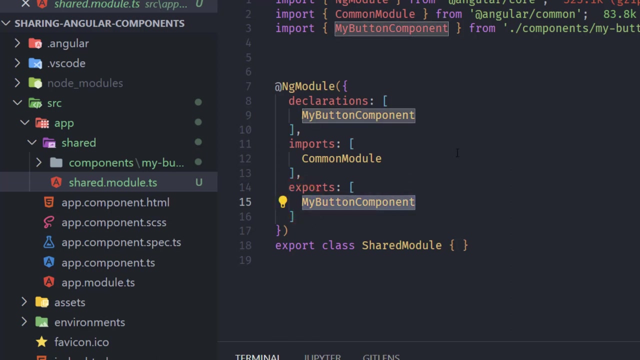 component is going to be exported from shared module here. so we now now, as you can see, we have a components folder here, we have my button here component and in our shared module here we can see exports here and my button component here, as well as in declarations. so this means basically that this component is. 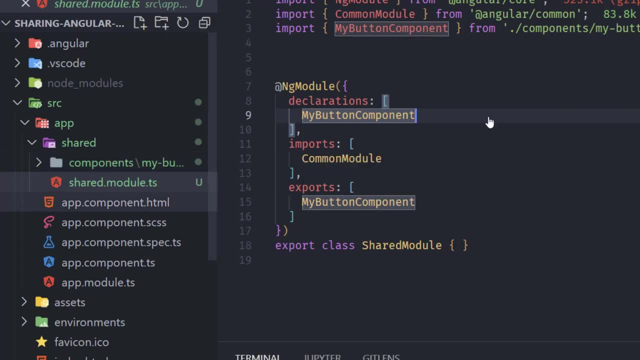 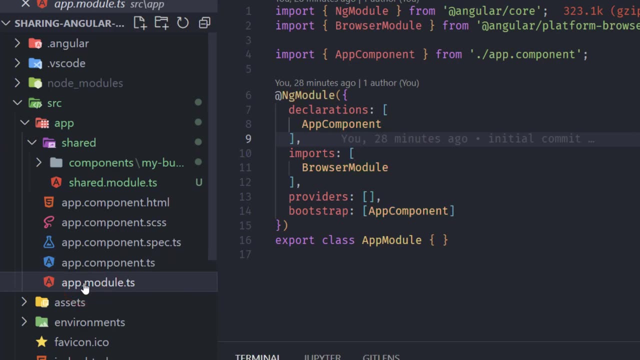 exported from our module. so when we have to use this component in any other module, we have to import the module only, as we are going to do right now. so in our app module TS we're going to import. here, next to the browser module, I will add shared module. 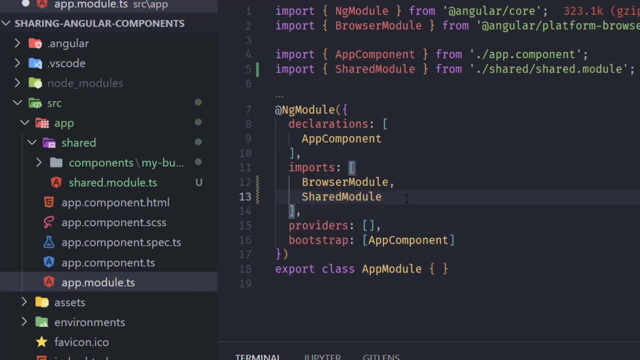 했어요. module hit, enter and importance share model save and that it so. now we have shared module imported and in this share module every single component that extruded is going to be available for us to use in our app module or any other model. so we are basically sharing components from mutual to a model. so in 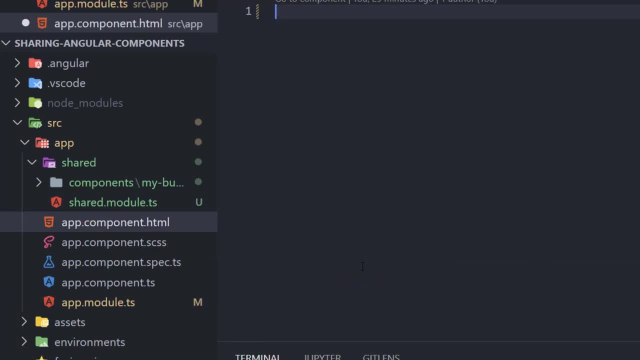 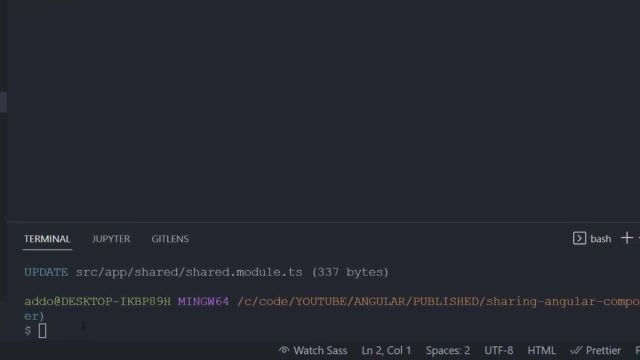 our app component. i'm up, remove everything from here, and now i'm gonna add up my button. that's my component here right now, so i'll just go to terminal ng s and dash, dash o. that means that it will open our browser after compiling this code, so we have to wait for it, but uh. 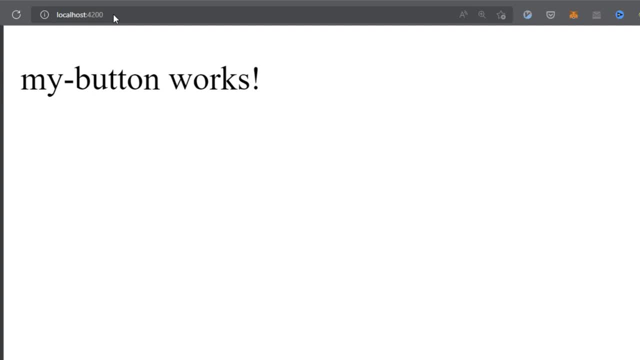 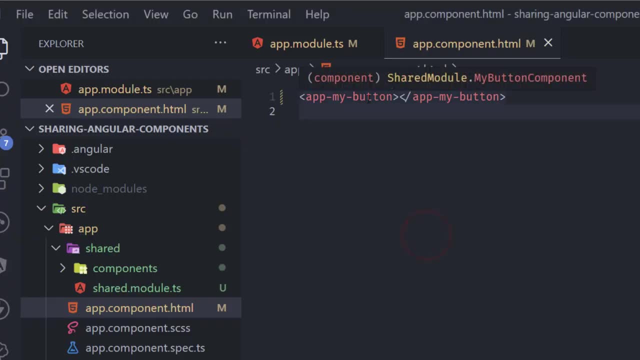 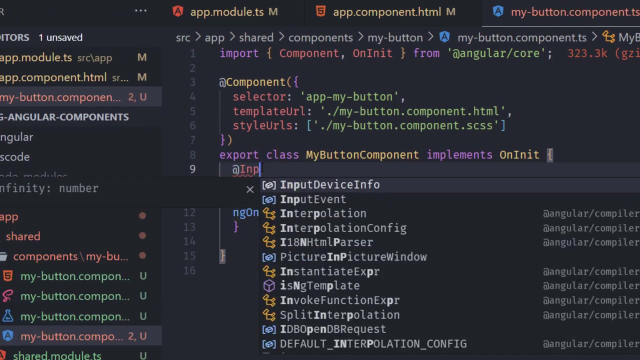 right now we can see here on port 4200 my button works, so that means that our component works. in our app component we could add something here to try this out. so in our my button component here i'm going to add at input, and this input is going to be imported from angular core, so add it here. 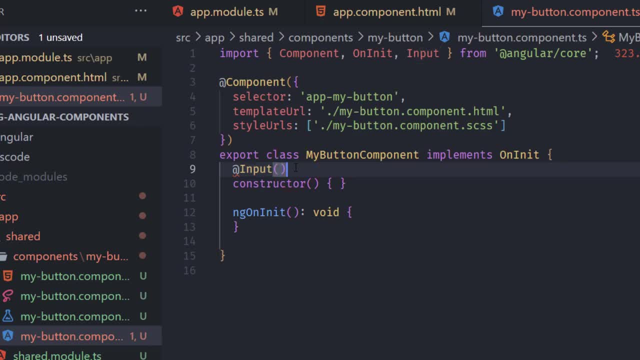 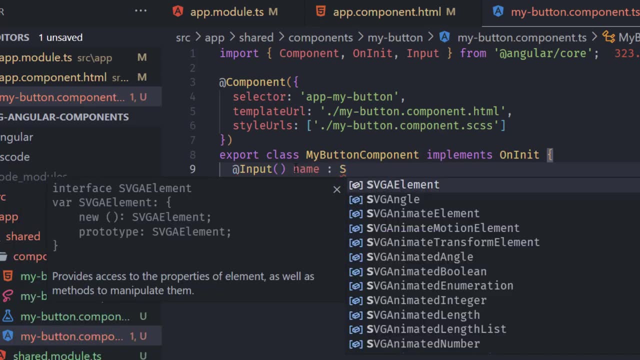 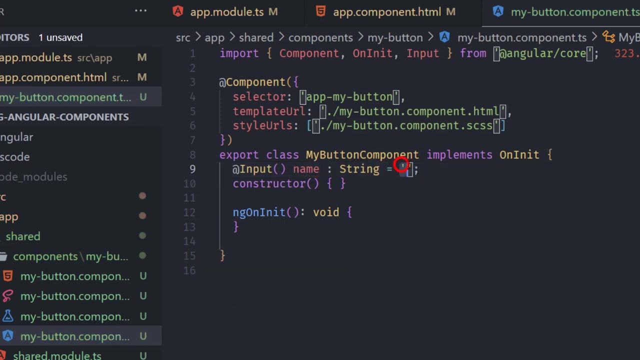 input and right now here i'll add a component named name. that is a type of string and we're going just to add as a fallback, empty, empty quotes here, single quotes. so if we don't add anything, it will just be empty. uh, after doing this, uh, we're going to, we're going to use our name here in our my button here. so instead of paragraph here,